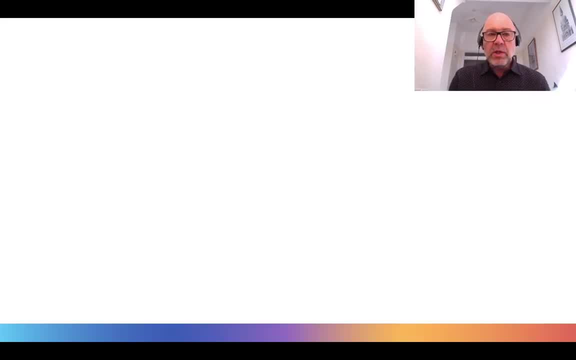 So a primary distinction with the NSSEC are between employers, people who buy the labour of others and have some degree of authority and control over them, The self-employed or own account workers, who neither sell their own labour or buy the labour of others, And employees who sell their labour to employers and in doing so put themselves under the authority of those employers. 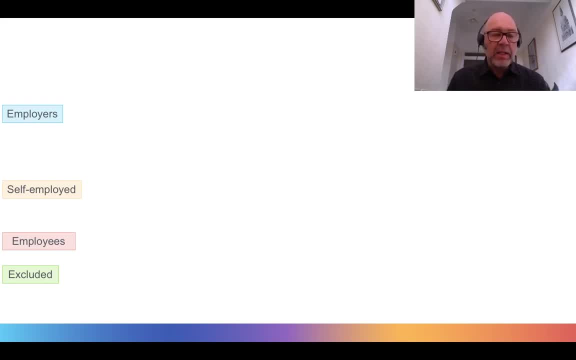 And about. you know, a high 80% of people in the workforce are employees, and so obviously they're not a unified class in an official dataset, And so obviously they're not a unified class in an official dataset. And so obviously they're not a unified class in an official dataset. 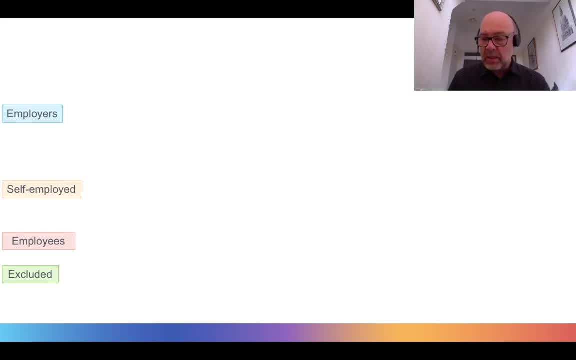 of themselves, and so there's a way of distinguishing between that which I'll get into, and then also within the NSSEC, there is a place for those excluded from the workforce, such as the long-term unemployed and those who've never worked, but we'll go into more detail in these. there's no ideal way of going about. 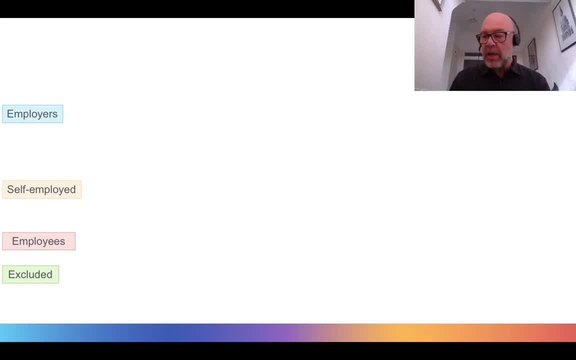 which order, because some overlap with others. but if you bear with me, I'll try and flag up when I'll deal with an issue in in greater detail later. so if we deal with employers first, in the NSSEC we distinguish between employers of in large establishments and small establishments and pragmatically this is: 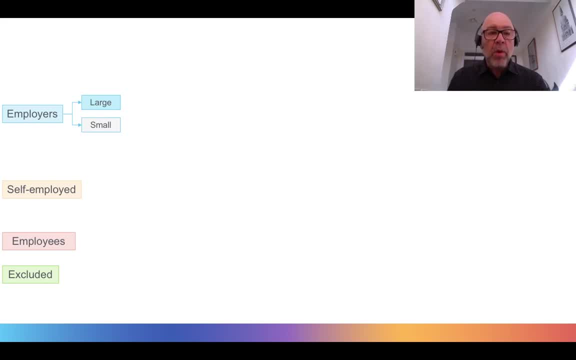 using a cutoff of 25 or more employees for large and less than 25 for small. but there's an exception here and this exception runs pretty much across all of the, whether it's in employers, self-employed employees and manager or status and that sort of thing. and that is if you're a if, if the high 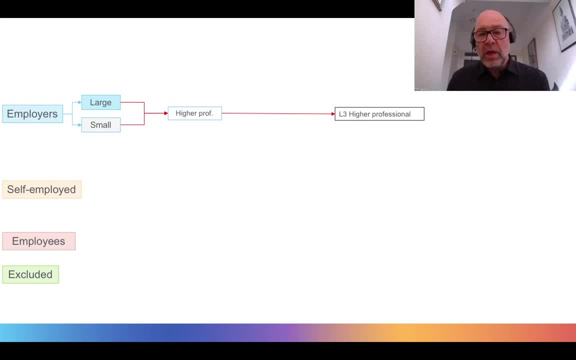 professional occupations always just go to higher professional occupations, and so we would say: a professional is a professional, is a professional, and so that overrides the other, the other status, and this is because, you know, empirically we find that there's sometimes the borders between self-employment and employment. 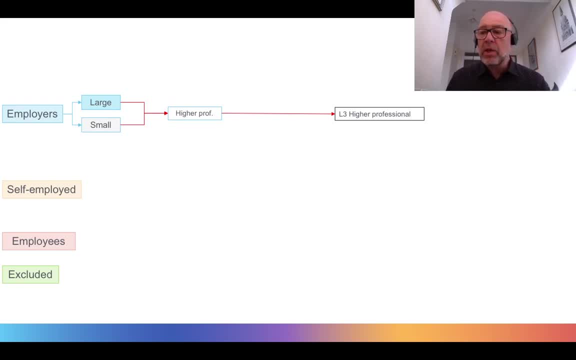 for professionals are hard to distinguish, and other times it's particularly in regard to managerial status, the you have to be a professional to be a manager in that profession first, and so that we we've determined that that's the one that takes priority. so for large employers we- you can see here that lower professionals go into- 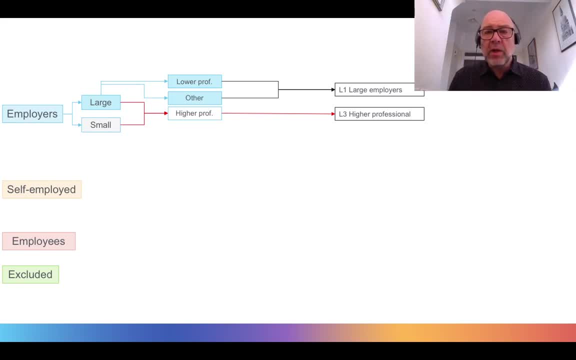 the operational category of large employers, as does every other occupation. as a little note, here you see the l1 and the l3- l you could means long form or these are our operational categories- who are then clustered together to form classes which i'll get onto later. so we see for lower professionals. 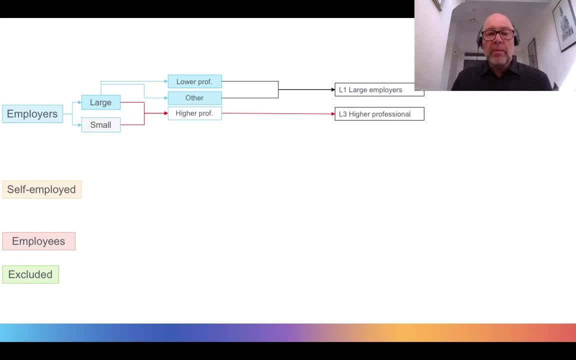 that, being a large employer, an employer in a large establishment takes precedence over the lower professional occupations. I'll get into the distinguish the the differences between higher professional occupations and no professional occupations when we get to employees, and similarly for employers in small establishments, apart from lower professionals, which do go to l4, which is the lower professional operational. 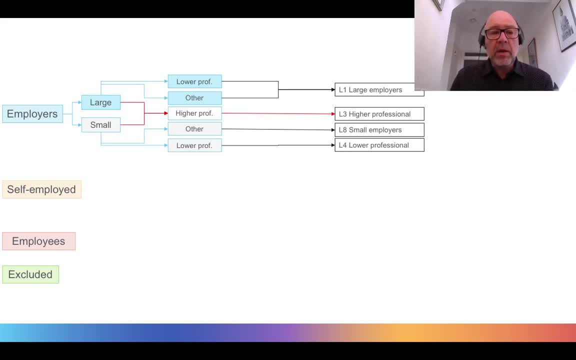 category that's that takes precedent over being a an employer in a smaller session and all others go to l8, which is this the operational category for in small employers, if we move on to the self-employed or in the camp workers. as we said, professionals are professionals. 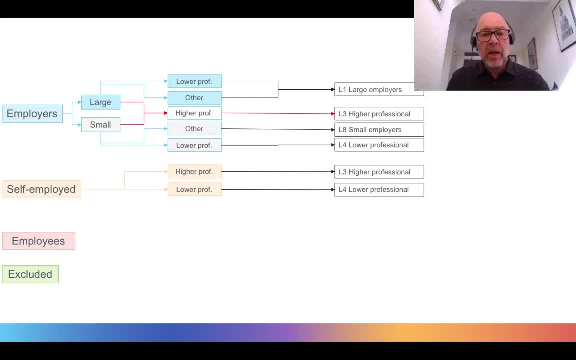 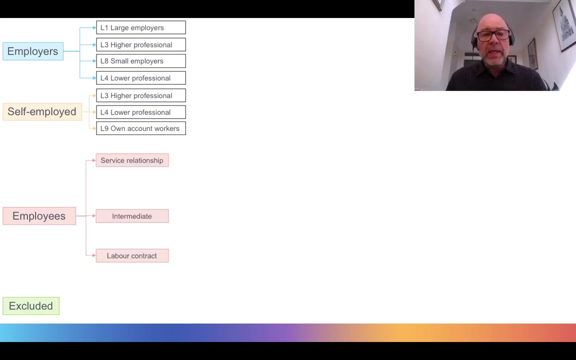 so higher professionals stay that way, lower professionals stay that way and everybody else who's a self-employed goes to l9, which is an account workers. now i'm just gonna shuffle this slide around to give me a bit more space to deal with employees now within the NSSEC. 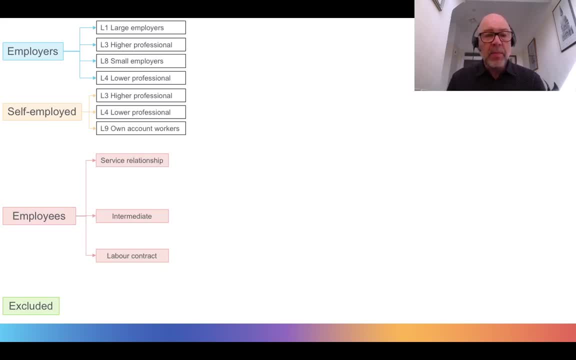 obviously not all employees are treating the same, and there we identify three basic types: a service relationship, an intermediate form of relationship with the employer and a labor contract. so these broad three positions are how employees are generally regulated by their employers through their employment contracts. and so first the 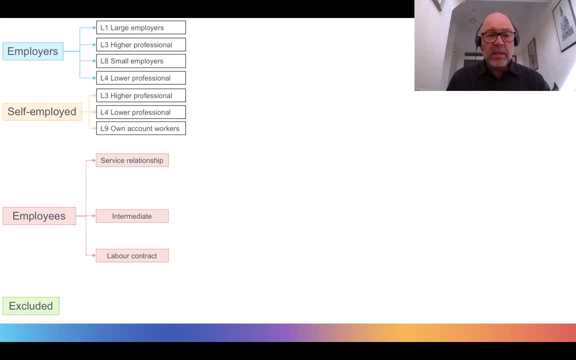 service relationship. this tends to be typified by employees providing a service for compensation. compensation is usually a salary. it's usually involving a long-term employment contract, and these are likely to exist where employees exercise delegated authority for the employers. they have specialised knowledge and expertise and they use them in pursuit of the employers goals. 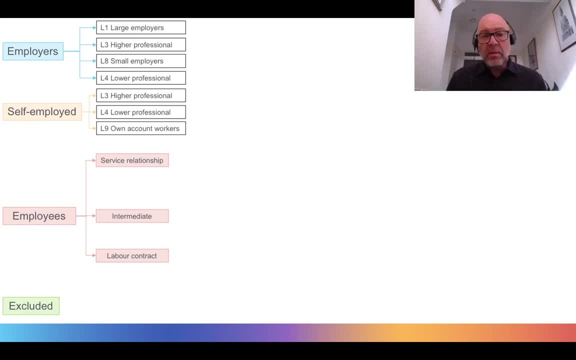 and missions of the organization, and this inherently entails a certain amount of autonomy and discretion for the employee, and these are typically found in higher professional, senior administration and senior management occupations. there's a more restricted or attenuated form of the service relationship, and this is where we distinguish between higher professionals. 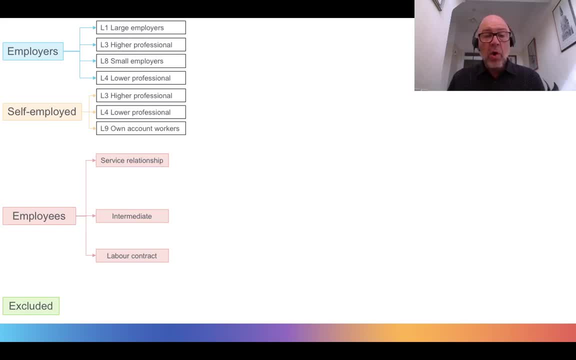 professional occupations and lower professional occupations, or between higher managerial occupations and lower managerial occupational occupations and higher technical occupations. in that we still we still think that there's a service relationship there, but it's not necessarily a service relationship. it's. it's not. it's in an attenuated form compared to: to the higher, the higher. 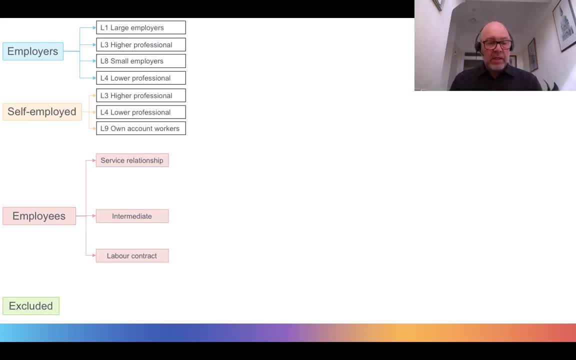 occupations. in contrast to this stands the labor contract, which is usually a relatively short term exchange of money for effort. usually employees are closely supervised and pays typically for the amount of work done, all the time worked. these are usually found in what historically we've called working-class occupations, but there's an attenuated 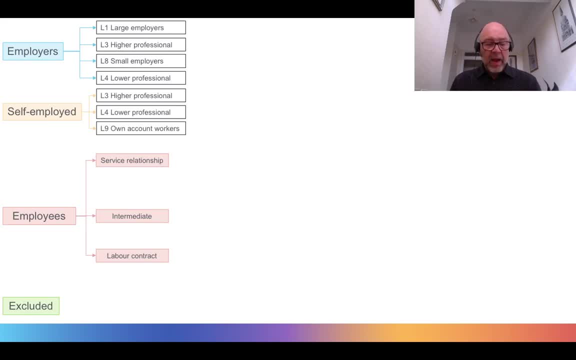 form of this also, which is found for supervisors and skilled workers normally, and the intermediate or the mixed form of employment relations combines aspects of the service relationship and of the labor contract, and these are typical in clerical and some technical and sales and service occupations. now, if we see, 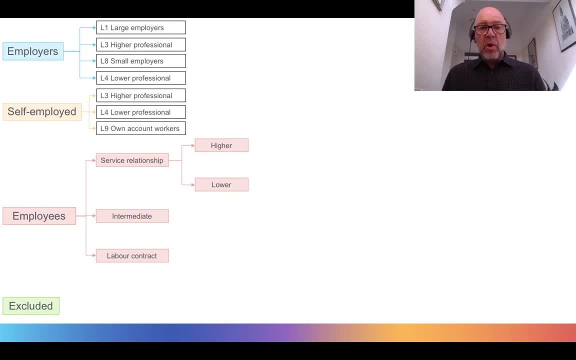 how these then go, work through to the operational categories for the NSSC see. so the service relationship will split that between higher and lower, or a full service relationship and a more attenuated form a bit and you see, for managers, higher managerial occupations goes to L, to professionals, as before L3, and for more, 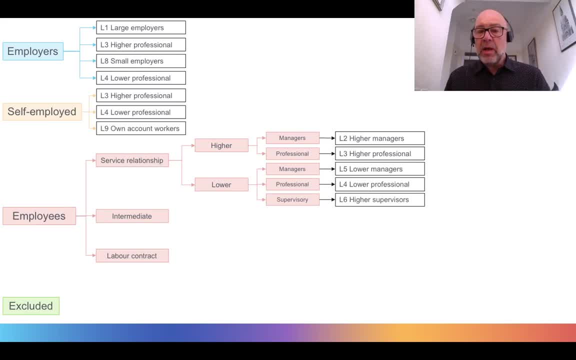 service relationships: lower managerial occupationals go to five, lower professional occupationals to four, and then higher supervisors. they they go to l6 and and the supervisors in l6 normally super, supervise employees who have an intermediate form of employment relationships and they here are in l7. 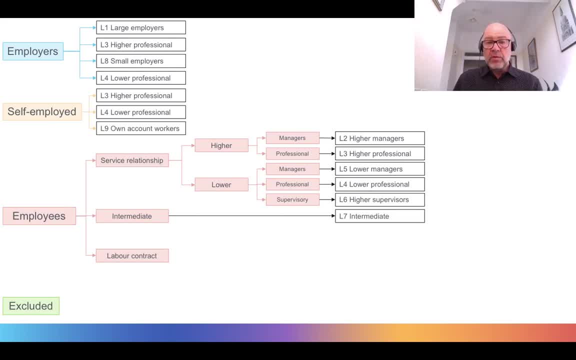 so the employees are in l7 and their supervisors are in l6. within the labor contract we, the NSSEC, split out into supervisory occupations so these have an attenuated labor contract. so they have some more aspect, some smaller aspects of the service relationship within that. so they go to l10, which is lower supervisors and 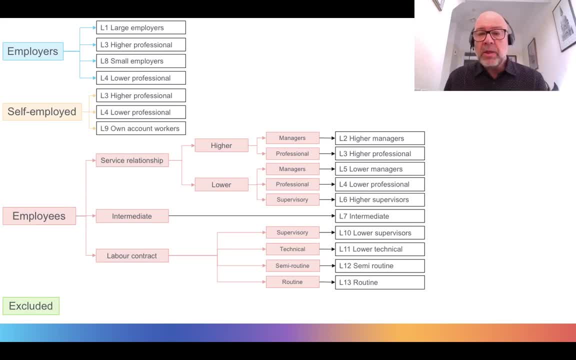 then there are technical occupations, lower technical occupations, higher technical occupations go in l4, and then there are semi routine and routine occupations which go in l12 and 13, and sometimes you can operationalize for the NSSEC, the never worked and the unemployed, which go to l14. now, if I just 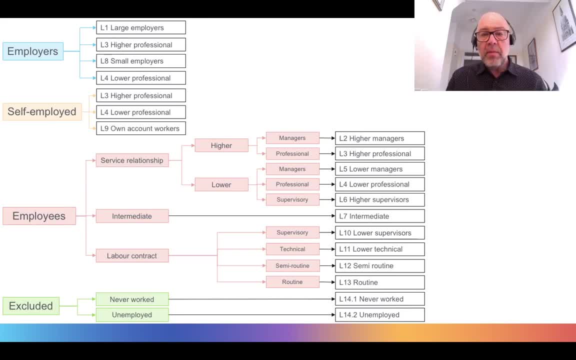 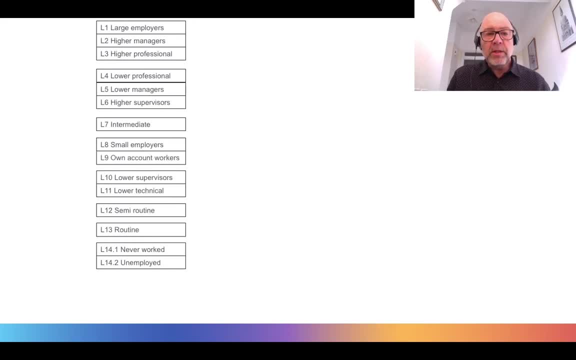 tidy up this slide. I hope that it will will remove the duplicates and then, if we order them, we can see how the operational categories then cluster into the different classes. now the NSSEC is a different category. so we can see how the operational categories then cluster into the different classes. now the NSSEC is a 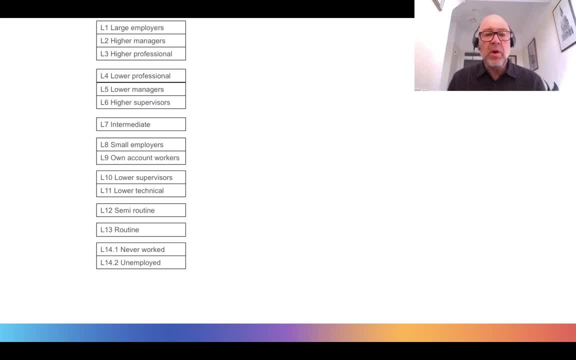 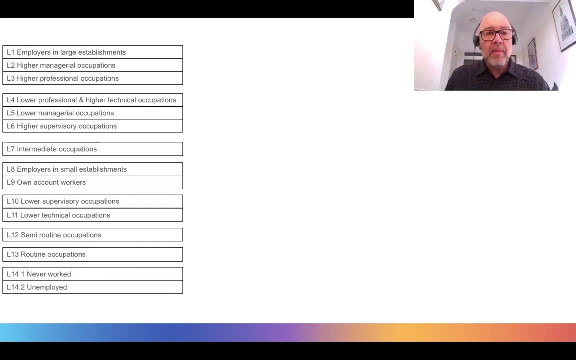 SOHA긴. so there is the eight-class version, which clusters in this way. this is the one that's been adopted by the office for national statisticsMAEAITSUM zw peuvent, adopted by the office for national statistics as the official NSSEC. and sometimes class one is split into class 1.1, which is employers, and 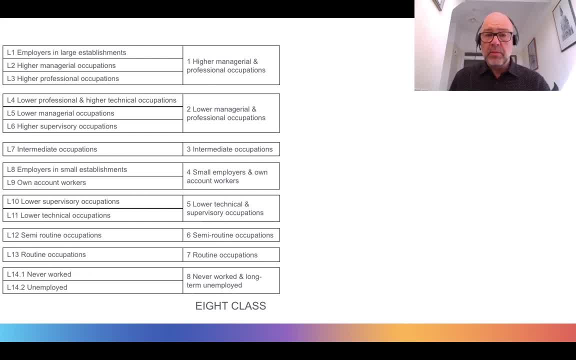 managers, and then 1.2, which is higher professionals. sometimes you see 1.1 and 1.2, but it's just a splitting out of of class one in the a class version. sometimes class eight can't be operationalized in your data sets. it depends on what you've got there. but because it's nested, 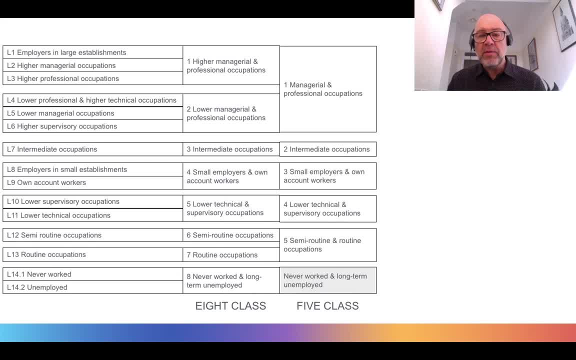 the NSSEC can be collapsed into a 5 class version where there's no distinction between higher and lower managerial and professional occupations and semi routine and routine occupations are clustered together and, going one step further, there is a 3 class version which clusters the lower technical and supervisor occupations with the lower technical and super 51 subкомmunities. 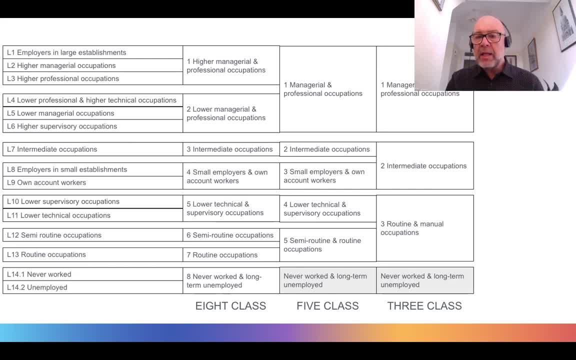 the routine amount with the route semi routine and routine, and the intermediate and small employers and own account workers clustered into class two. you have to remember with the NSSE see that it is a nominal classification. although we use one, two, three, four, five it's, it's not considered ordinal because 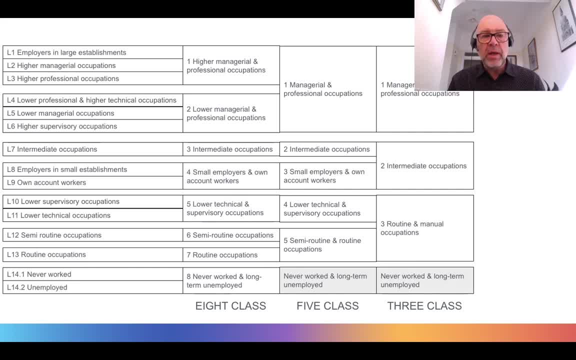 particularly because of the self-employed in class four, in the eight class version. there is some argument that the three class version can could be considered ordinal, but there's a debate on both sides of that. so the what covered here is how we get from the conceptual basis of the NSSE. 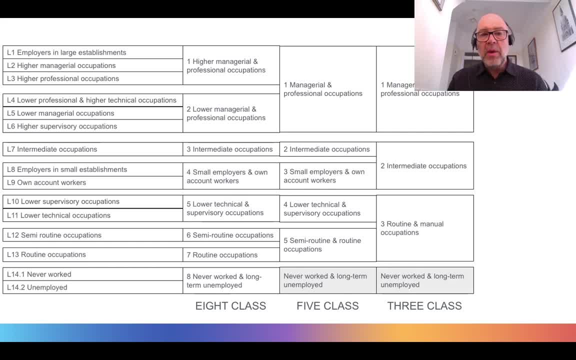 seeing to regard of employment relations through to the operational categories and then through to the different version, different analytic class versions of it. if, if you're looking back maybe at the 2010 version of the NSSE, see in the operational categories instead of just seeing l1. 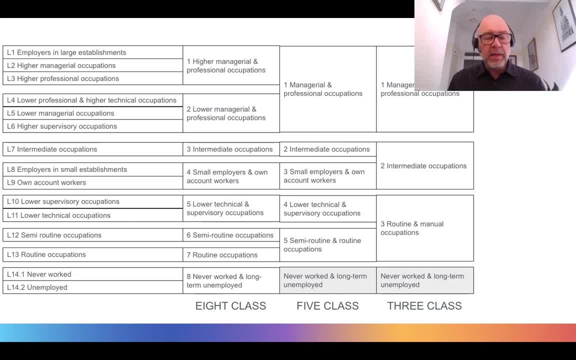 through 13, you might see some likes, particularly in, let's say, three or four class versions of the NSSE. see in the operational categories. instead of just seeing l1 through 13, you might see some likes, particularly in, say, 13, you'll see l, 13.1, 13.2 and they are operational subcategories. these were 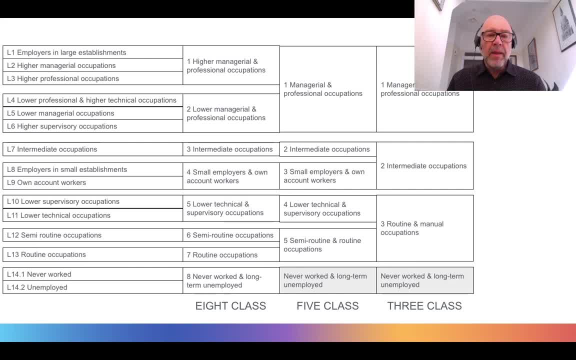 dropped for the 2020 version. they were originally put in in 2000 to help link back to the former classifications- social classifications- but in rebasing for 2020, we decided that it was no longer feasible to maintain these, and so now we just have l1 through 13 for the 2020 version. 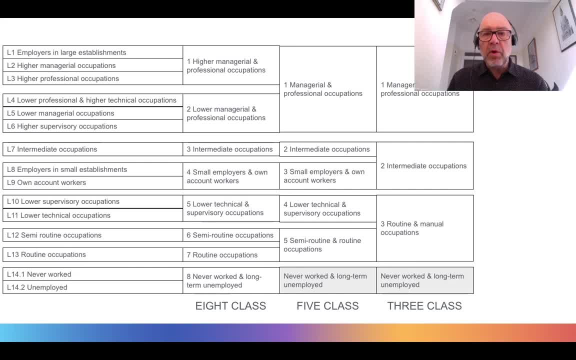 the employment ones within within the NSSE see. as I said a bit earlier there's. I'm going to do a small supplemental on how to actually put the NSSE see derivation matrices on your data set and what information you have to have, what variables you have to have. this is detailed in quite some depth in the 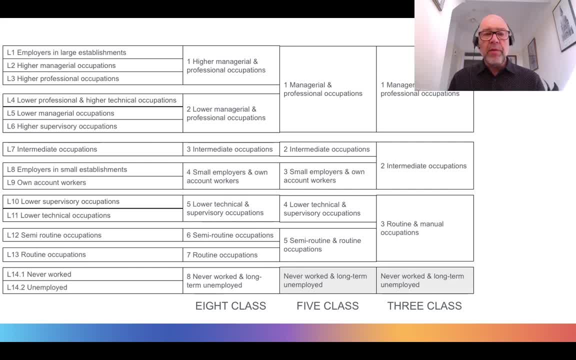 standard occupational classification, volume 3, which is available online, and also there is a report there which details how we rebased the NSSE see for the 2020 version of of sock in preparation for the census in 2021. anyway, good luck with that and I'll see you at the in the supplemental.